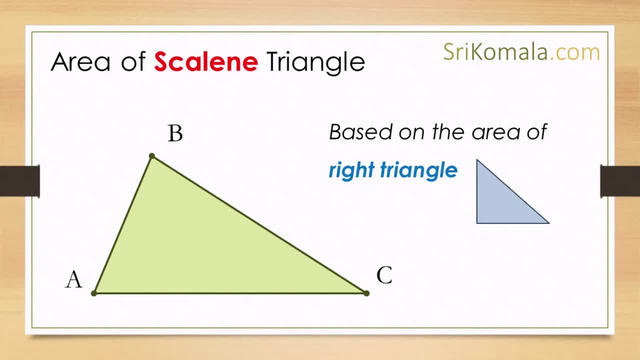 of the area of triangle is a half of its base times its height. The area of triangle is based on that of right triangle. The proof of the area of right triangle are provided in our previous videos. Please find the links to the previous video somewhere. 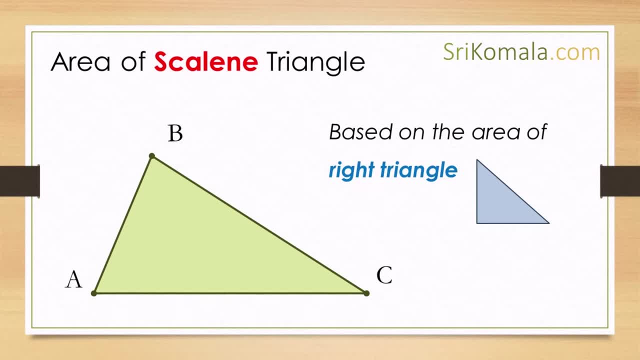 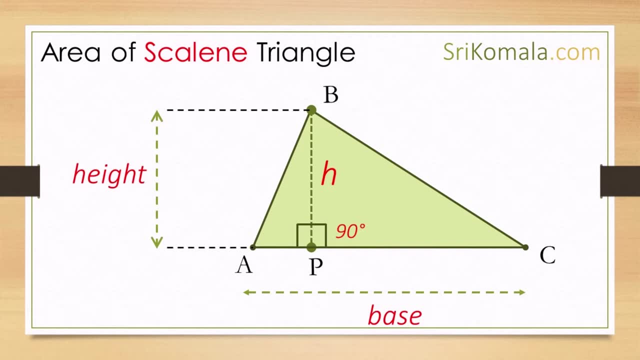 on the screen or in the description below. First of all, we need to acknowledge that the height of triangle must be perpendicular to its base, And the height of triangle must be perpendicular to its base And the 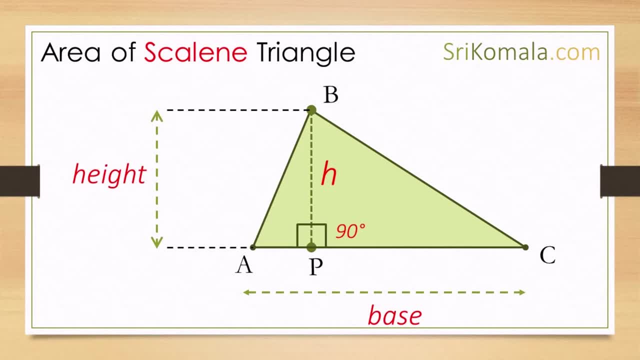 height of triangle must be perpendicular to its base And it must be connected to one of its edge. Here, as shown in the figure, the height of the triangle is expressed as line h And it connects edge b and point p on the base. Next let us divide. 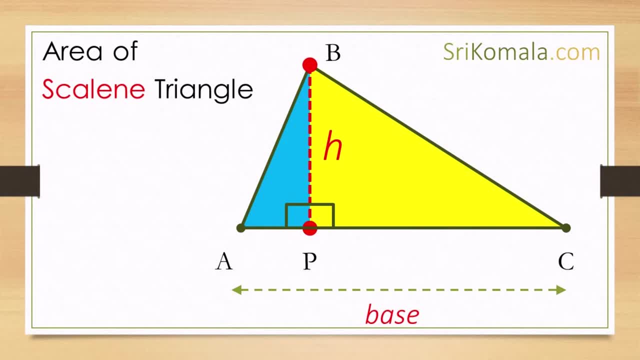 the triangle a, b, c into two smaller triangles. Next, let us divide the triangle a, b, c into two smaller triangles And the height of triangle is based on the height of triangle a, b, c and point p. Those are triangle. 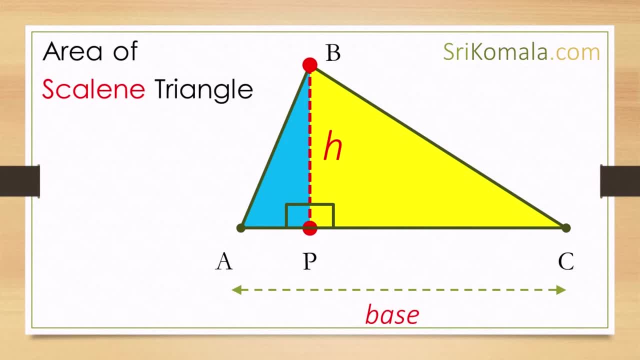 a, b, p, which is on the left side of line h, Shown in the figure, as the blue right triangle And triangle b, c, p, which is on the right side of line h, Shown in the. 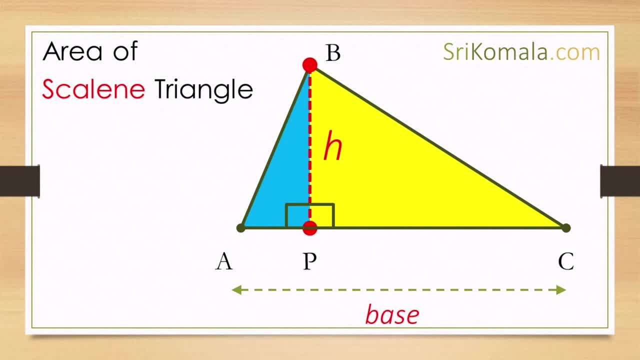 figure as the yellow right triangle. Both triangle possess a, b, c and point p. Those часть triangles are classified as r, nossas right angle, or ninety degree angle, which is located on point p. Therefore, both triangle are classified as right triangle. 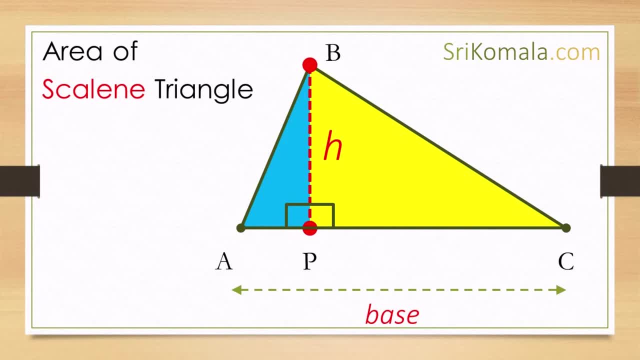 Please also notice that the base of the scaling triangle is represented by the line a, c And the point p is located on it. Hence, here the area ofocyst. here is the area of facebook, And hot spot is at block. This image is to be shown as above. Here the exists in the vertical line. below that are the direction of point p, which is located on point c. The area of this triangle isath working, which is located on the position of point p, which is located on point p. thus it can be slightly. 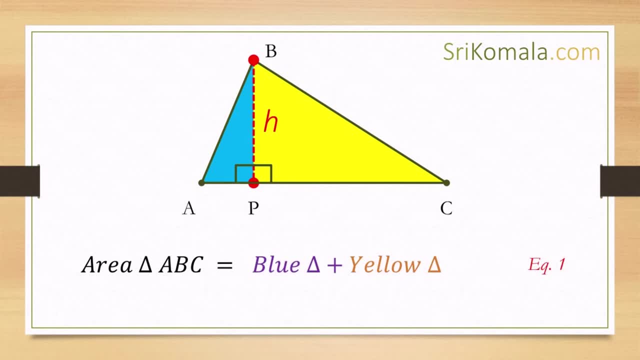 askew, Then later we can see the base of the 변 en the in line ansigh asthenly centers hanged aroundational. hence the area of the scalene triangle can be expressed as the addition of the. 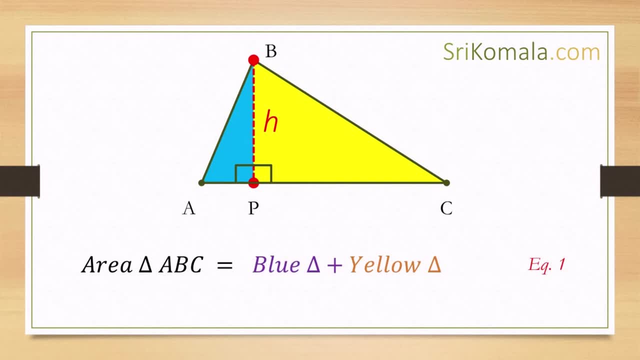 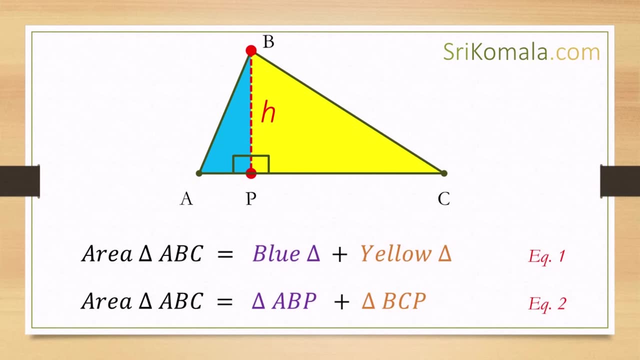 blue triangle and the yellow triangle, as shown in equation 1.. in other words, the area of scalene triangle ay b- c can be expressed as the addition of the area of right triangle ay b- p and right triangle b- c- p, as shown in. 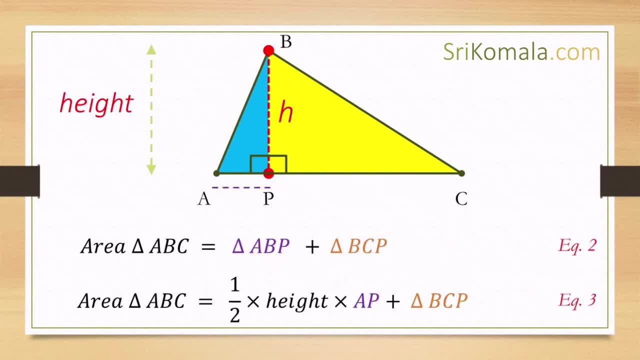 equation 2.. the area of the blue triangle or right triangle, ay b p can be expressed as a half of height times the length of ay p, as shown in equation 2.. 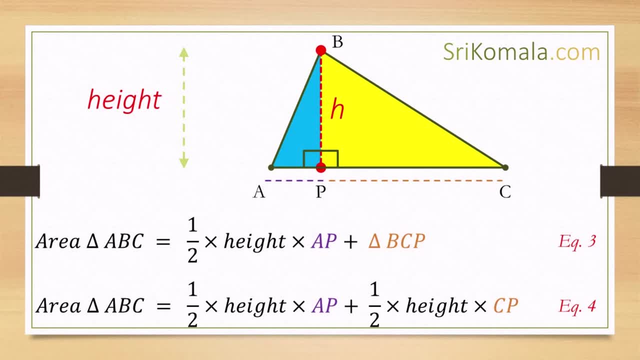 in other words the area of the yellow triangle or right triangle, b. c p can be expressed as a half of height times the length of c? p, as shown in equation 4.. 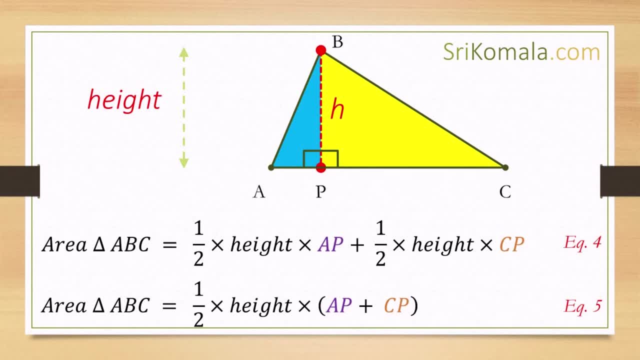 by utilizing the distributive property. the equation 4. of, according to the Meter, can be expressed as a half of height, as shown in equation 5.. the equation for glass and fry- reichting glass. 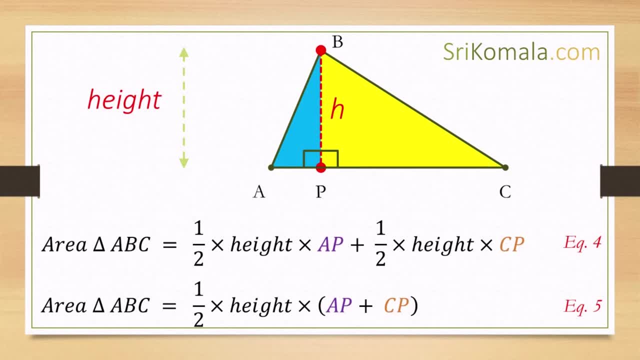 can be expressed as a half of height times ay p plus c p, as shown in equation 4.. click the link to the previous video explaining the distributive property somewhere on the monitor or in the description below. 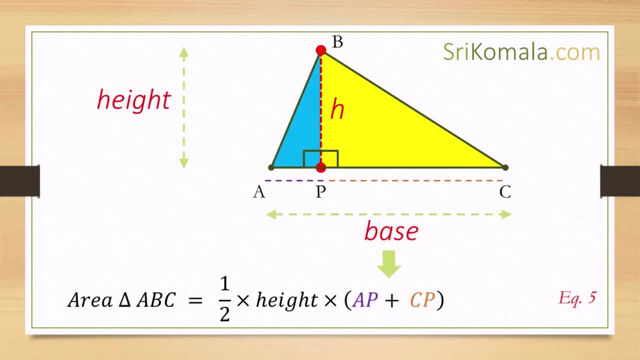 in equation 5.. the addition of ay p and c p can be expressed as a half of height times ay p plus c p, as shown in equation 5.. 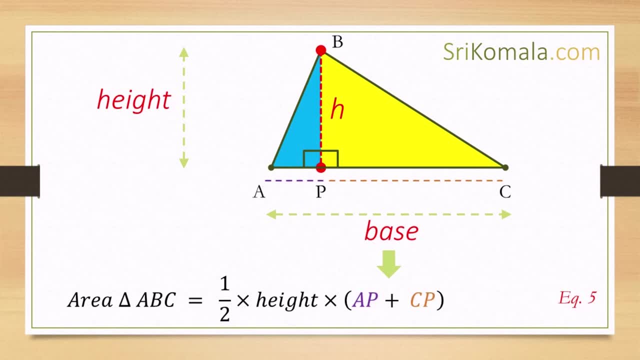 b and c. p is actually the base of the scalene triangle ay b, c. thus equation 5, can be expressed as equation 6.. where, as the area of scalene triangle ay b, c is a half of height times base.